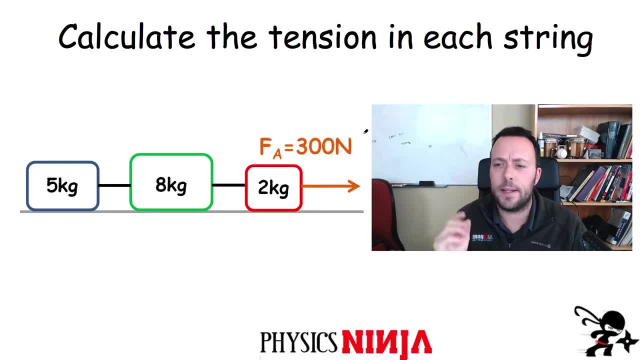 Hi everybody, Physics Ninja here Today we got a nice little problem for you. We just want to calculate the tension in each string. So I have three blocks: five kilograms, eight kilograms and two kilograms- And I'm pulling kind of on the end here with an applied force. 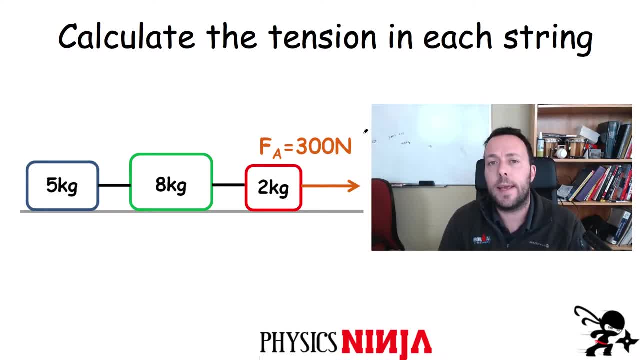 equal to 300 newtons. So let's go see how we calculate the tension and the tension here between blocks five and eight, And also how do you calculate the tension between blocks eight kilograms and two kilograms. Let me show you how to set it up. do free body diagrams? 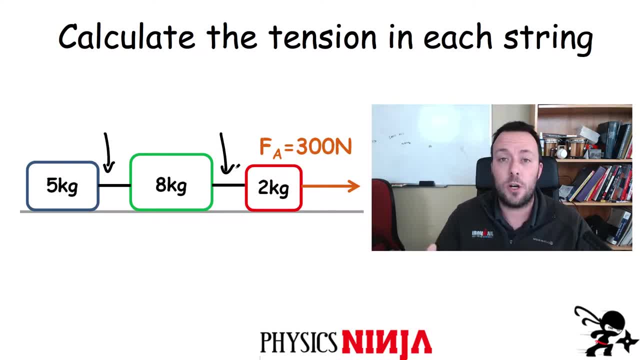 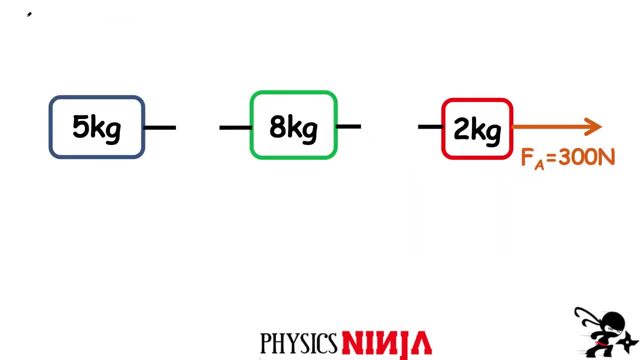 write down Newton's second law for this problem and then solve to obtain the tensions for each rope. All right, let's get started. Okay, to set this problem up here. what we're first going to do here is we're going to label them. This block here is going to be M1.. This block 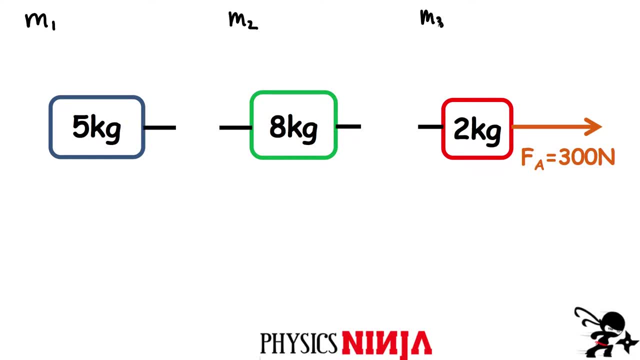 here is M2 and its value is eight kilograms And this block three is going to have a mass- M3, which is two kilograms. So we want to label all the forces acting on all the three blocks. So we're going to start with the easy forces. We have the weight. This one is M1G. This 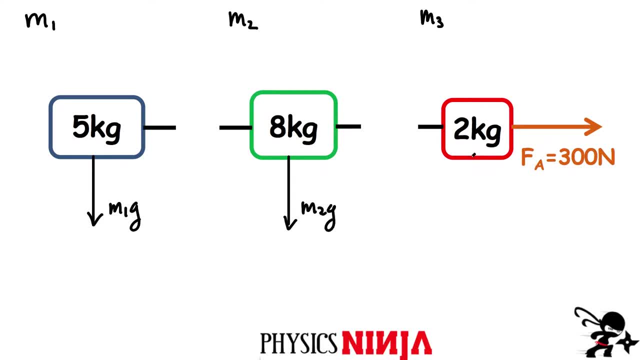 one here has a weight which is a little bit bigger. This is M2G, And the last one over here, since it has a mass M3, the force of gravity on this block is M3 multiplied by little g. Also for this problem, just to keep the math a little bit simpler, rather than 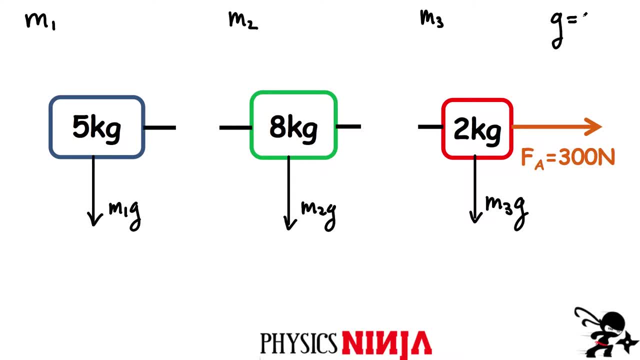 using 9.8 for the acceleration due to gravity. what we're going to use here, we're just going to use 10 meters per second squared, just for this particular example. Now, these three blocks were sliding across a table. Therefore, there is a force from 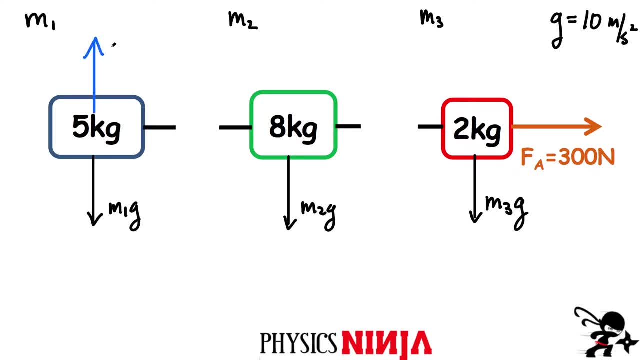 the table acting on each block, and you typically call those a normal force. I'm going to call this normal force N1.. The normal force acting on block M2 is going to be N2.. Now, it's not necessarily the same as N1. So that's why I'm using the subscript here. one and two. 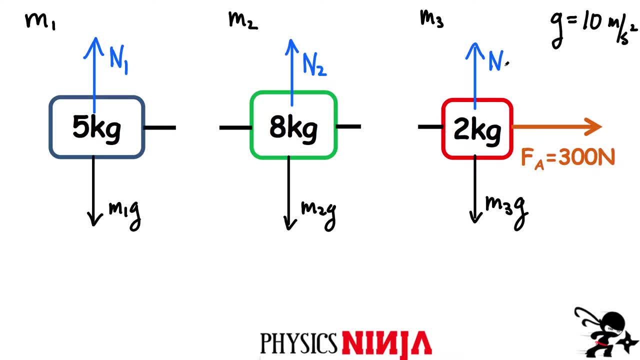 And likewise here, this one here, the normal force acting on the two kilogram block. I'm going to label that one N3.. All right, And the last one here is the weight. This one here is a mass M3.. This one here is a. 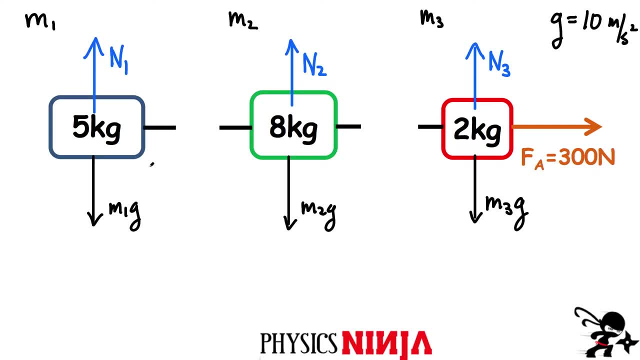 part now is actually the tension, which is really what I wanted to solve for, and actually I've cut the rope. so you can kind of get an indication now. if you look at this five kilogram block, there is a rope connected right here. if I look at the eight kilogram block, there's a rope connected right here, and to find 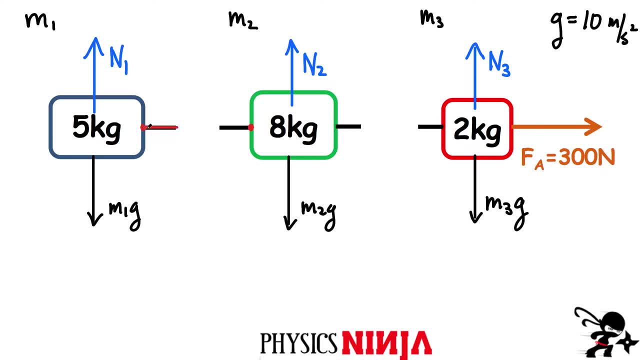 the direction of the tension. you just go from the connection point and you go follow the rope. so for this one here I'm going to call this tension t2, and over here on the eight kilogram block again, you start from that, where it's making contact with the eight kilogram block, and I just follow the rope. and now this: 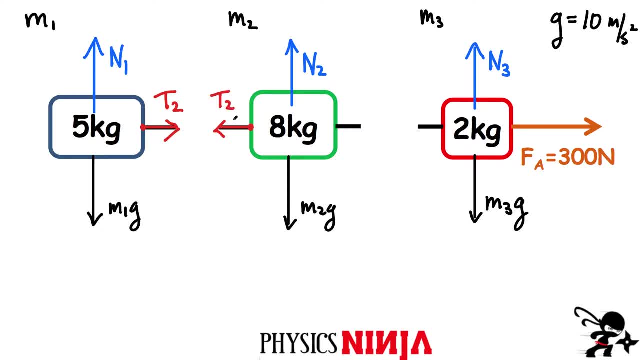 force here. t2 is going to be the same as this one, it's just in an opposite direction. okay, because it's connected and follows the rope. all right, there's one more we have to do. we can't forget about the string over here. so again it's. 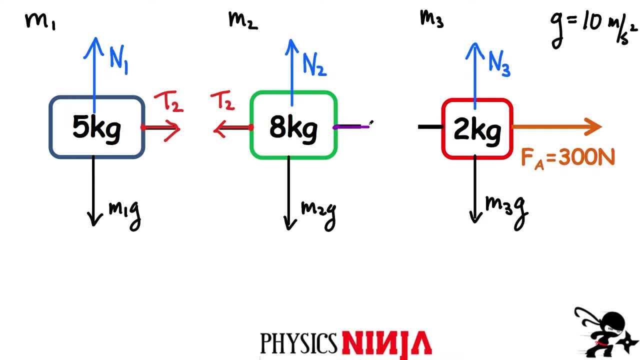 in contact with the eight kilogram block to find the direction. you simply follow the direction of the string, and this one here I'm gonna call it t1. so notice also that I have a different notation for the tension in this leading rope compared to the rope connecting the last two blocks, the 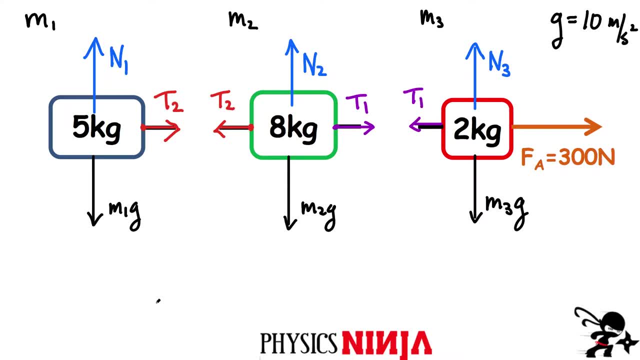 tension might end up being the same, but we're gonna let the physics kind of tell us whether or not it's going to be the same. all right, and that's it. and then I also have my applied force, and the applied force is only acting on the two. 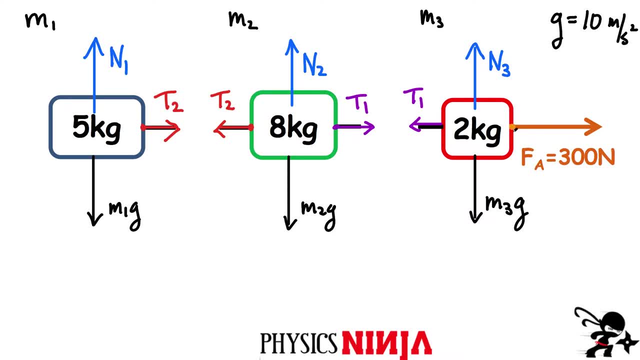 kilogram block, because I'm simply pulling on the two kilogram block. I'm not pulling on the eight or the five kilogram. so therefore, that is it. that is the free body diagram for this problem. the next thing we have to do now is we have to write down Newton's second law and 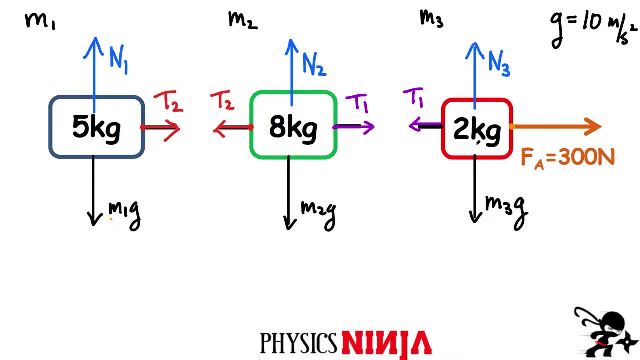 Newton's first law for each of these blocks and then solve for the unknowns. so let's go on the next page and do that, okay, before writing down Newton's second law for their, each one of these masses. what I'm going to do first is define a 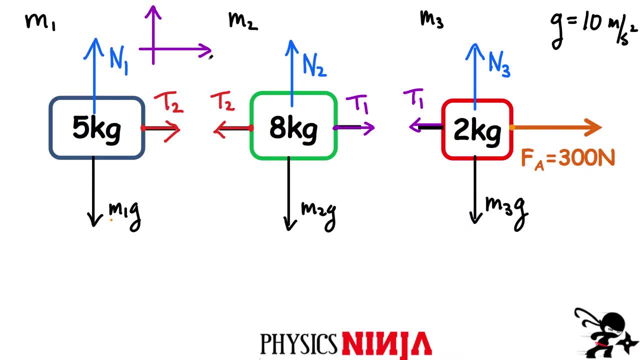 coordinate system. since we're adding vectors, we have to define which ones are going to be positive, which ones are going to be negative. so what I'm going to do is use, to use, the standard coordinate system. this is going to be my positive x-direction, and the direction that I'm going to be using is going to be: 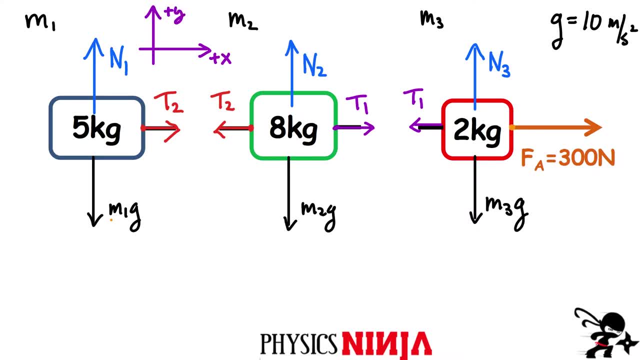 my positive y-direction. now what I'm really interested in now is the sum of the forces for each block acting in the x-direction. so we're gonna have to do that for each block and that has to be equal to the mass of the block multiplied by the acceleration of the block. so we have to do this actually for each block. 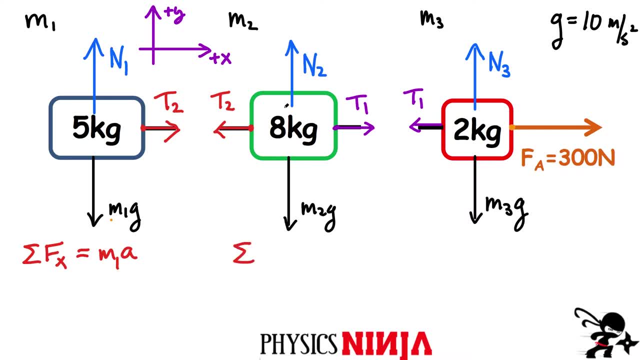 so actually I have to do this like this: I also have to write the sum of the forces acting on the eight kilogram block. that has to be equal to the mass m2 multiplied by the acceleration of that block, and I have to do the same thing. 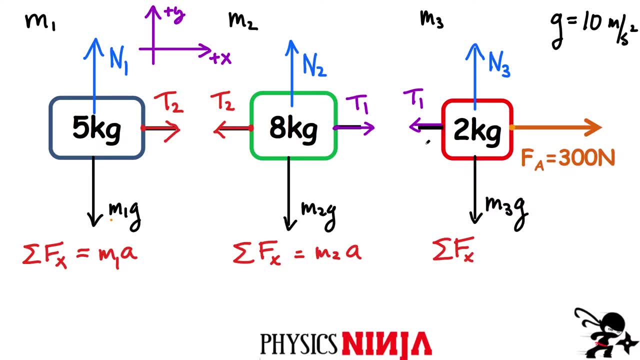 for the block, the two kilogram block, add all the forces in the x-direction and those have to be equal to the mass m3 multiplied by the acceleration. now, one thing you might have noticed over here is that when I wrote down Newton's second law is, I've actually set the acceleration to be equal to the same. 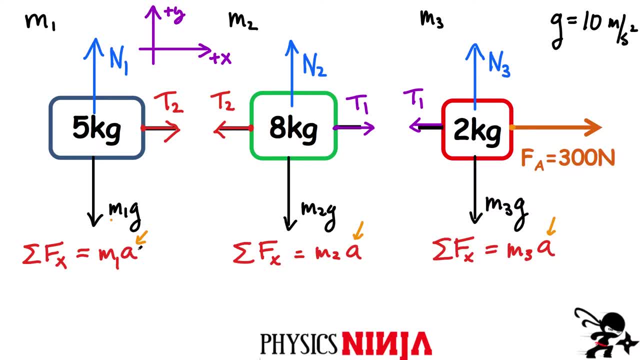 thing, and why have I done that? well, imagine if they're not the same thing. if they're not the same thing, it means that the blocks are going to slide farther apart or they're gonna get closer together. if they have different accelerations, okay, so they all have to have the same acceleration. that's really. 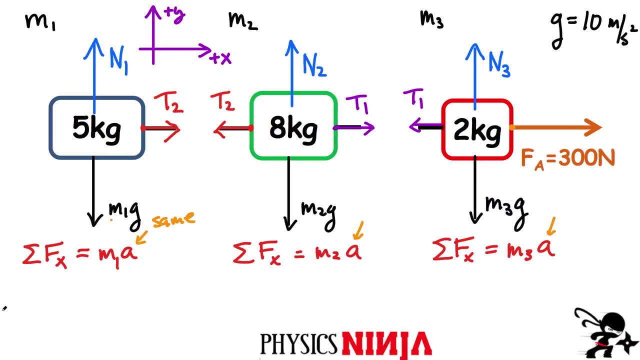 important, okay, so let's start off with the five kilogram block. I'm gonna call this equation one. let's look at all the forces in the x-direction acting on the five kilogram block. there's only one. this one's super easy. so you get tension. t2 has to be equal to the block m1 multiplied by the acceleration of. 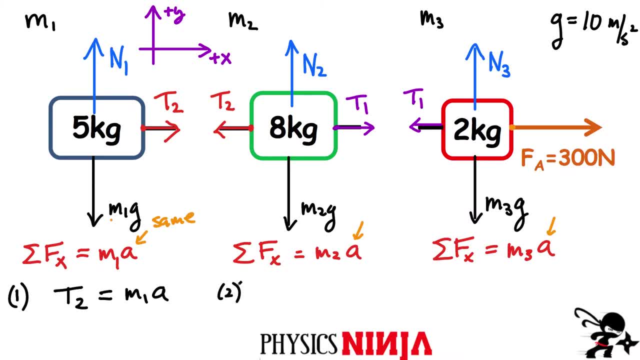 that block. that's equation one. let's look at all the forces acting on the eight kilogram block and again we're just focusing on the x-direction because we're looking to solve for tension. so notice, we have two forces here acting on the eight kilogram block. we have a 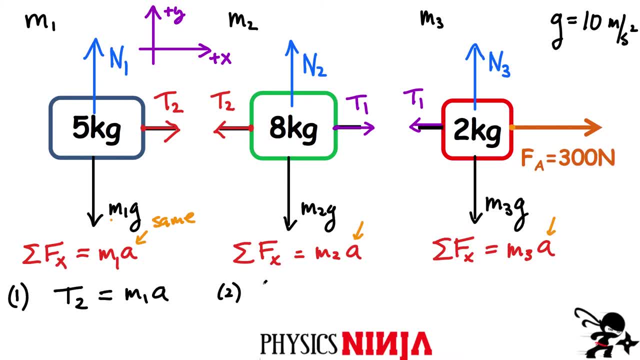 tension t1 and a tension t2. therefore, when I add all the forces, they should look like this: I should get positive t1, because t1 is pointing to the right, and negative t2, and it's negative because, according to this coordinate system, that force is pointing to the left. 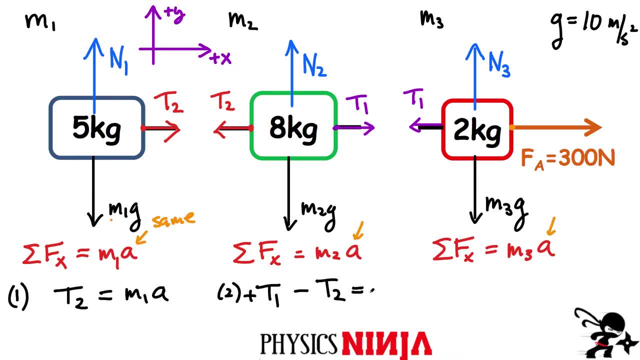 so I put a negative sign to indicate the direction. That has to be equal to m2a. alright, I've got two equations, let's do one more block, one more equation. we're going to call this equation three. Now, if I look at all the forces acting in the 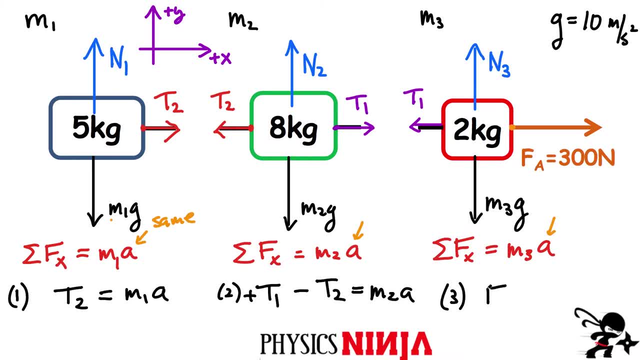 x-direction on this block. I should have something like this: my applied force, my 300 Newton's, pointing to the right. therefore it's a positive number minus the tension t1. and now I have negative here because it's pointing to the left. on the 2 kilogram block. 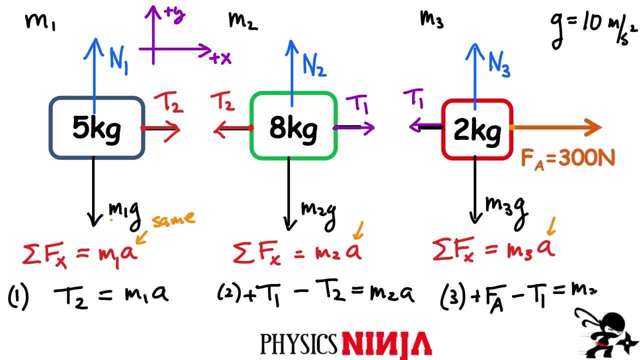 block And therefore that has to be equal to the mass of the block, M3 multiplied by the acceleration. So we have three equations over here and think about our three equations. What are the unknowns in these equations? Well, there's the tension, T1, and that's what 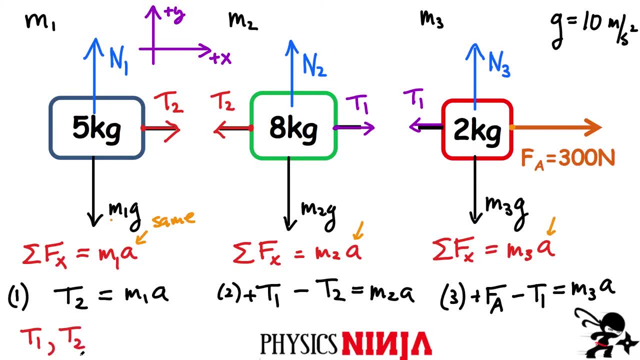 I want to solve, for I'm also looking to solve for the tension T2 and you're going to get something else out of it. You're also going to obtain the acceleration of the three blocks. So these are really the three unknowns. Luckily, I have three equations, therefore I can solve. 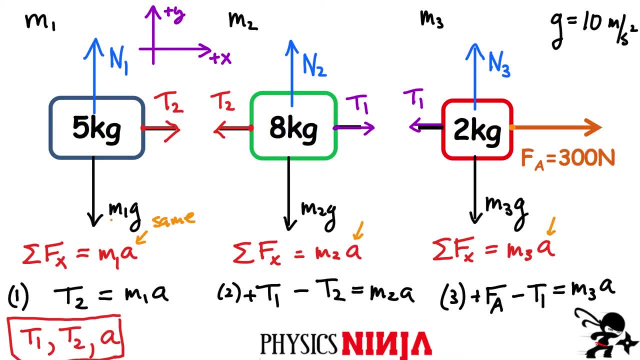 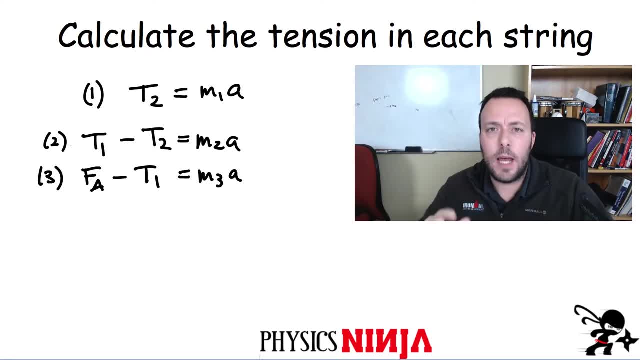 for those. So let's go on the next page and I'll show you how to set up the system of equations and how to solve this as efficiently as possible. All right, Hi, everybody. So this is what we have now. We have our three Newton's second law, one for each block, And I've rewritten. 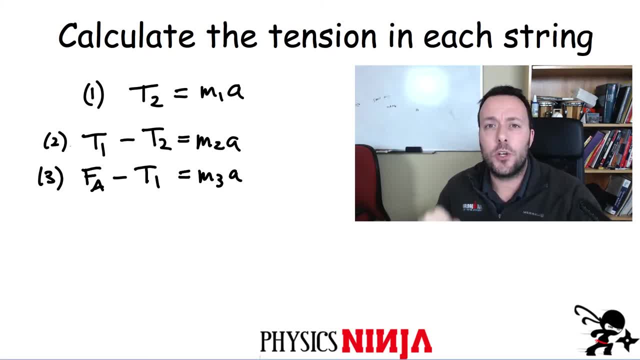 the three equations right here so you can have a look at them. Now I want to show you a really, really cool trick that you may not have realized. Now you could substitute the numbers in right away And then do a little bit of math: isolate and substitute in order to do that. But it's 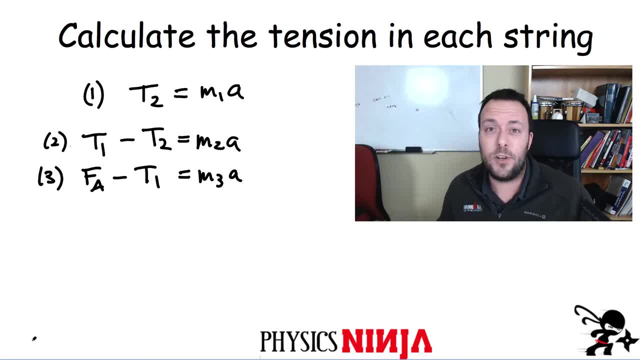 three equations right And three unknowns, So you'll end up having to do a little bit of work. I'm going to show you a little trick. This is kind of a pros trick. I don't want to give you all my tricks, but I'll give you this one here on how to obtain the answer. 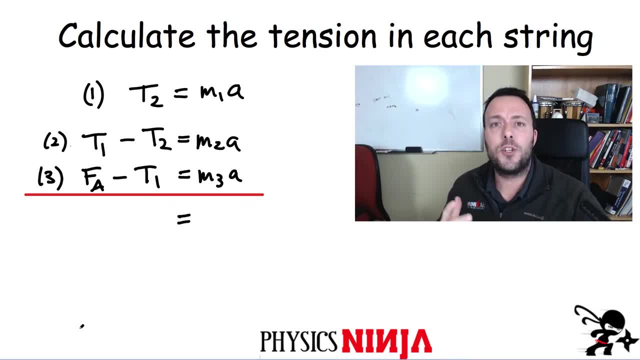 as quickly as possible. Actually, one thing I want you to notice here is that look at an equation one: the tension T2 is a positive number. However, in equation two, the tension T2 is a negative number. Have a look at the tension T1 in equation two. It's positive here, However in equation 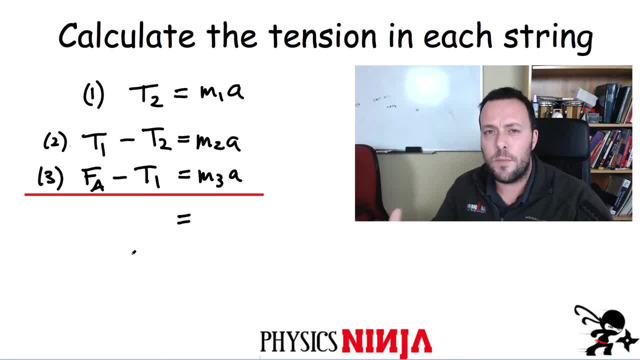 three. it's negative. So let's do something kind of cool. Let's add up the three equations. These are linear equations. You can solve them any way you want. One way to get rid of all these tensions is actually to add up the three equations. So if I do that, have 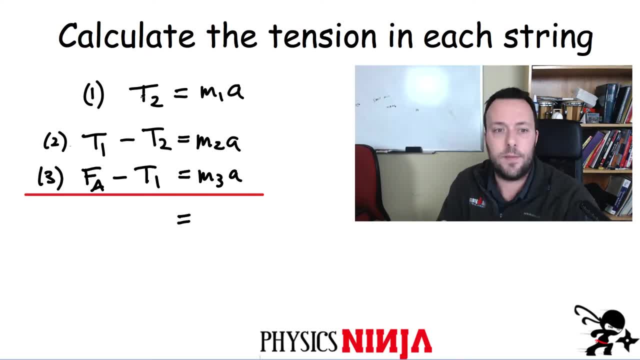 a look at what happens, So I won't have a tension T2.. That one's going to vanish, right? This one's going to cancel with that one, So forget about this. This will cancel with this one. The tension T1 is going to cancel with this one, And what we're going to be left with? 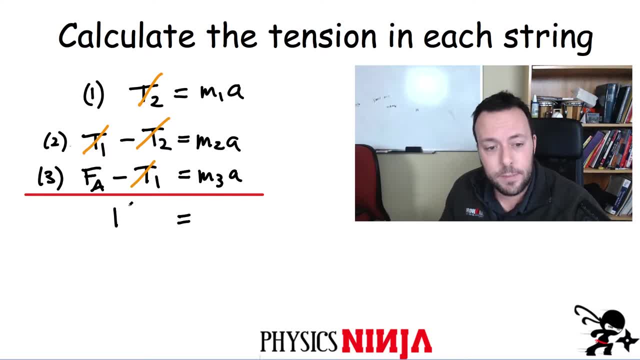 now at the end is simply on the left-hand side, is simply this applied force, which was 300 newtons. Have a look at what we have now on the right-hand side. Well, they all have the same acceleration and all I end up doing is simply adding up the three masses: m2 plus m3, multiplied by 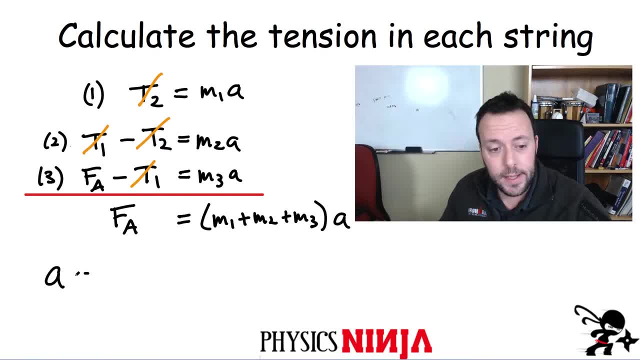 the acceleration. So, at the end of the day, what do I end up getting? That the acceleration is my applied force divided by the total mass of the system. It's as though all of those tensions have just vanished. So let's just write this down: m1 plus m2 plus m3.. And 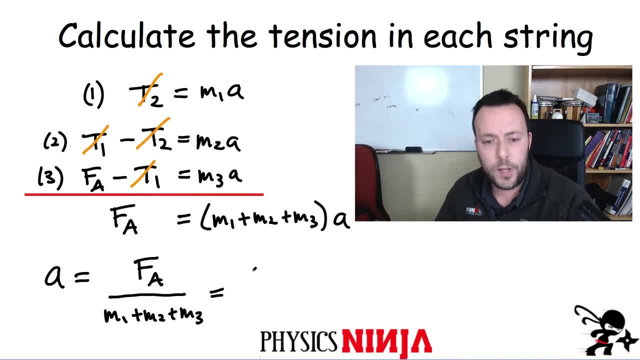 now we're going to substitute our values. So my applied force was 300 newtons. Now the blocks were 5 plus 8 kilograms plus 2 kilograms, So I'm left with 300 divided by 15. At the end I get a quite a big explosion. So I'm going to substitute 500 newtons for 500 newtons. 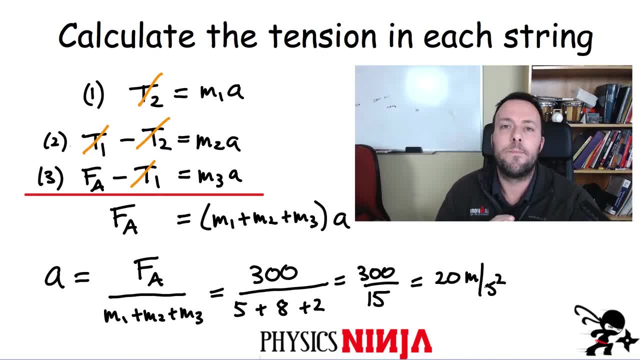 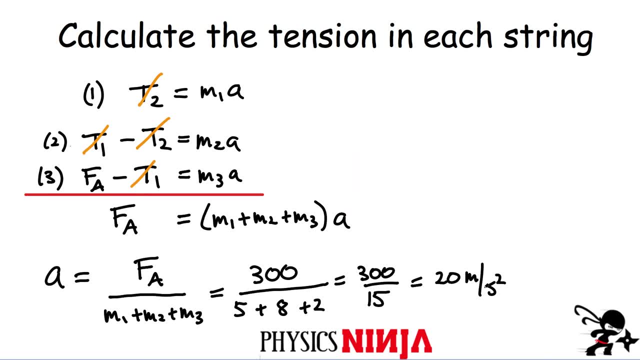 acceleration of 20 meters per second. squared, That's the acceleration. Now the goal was always to find what are the tension values between the blocks. So what we're going to do now is simply, if you go back to the equations that we had, look at equation one. Equation one simply says: 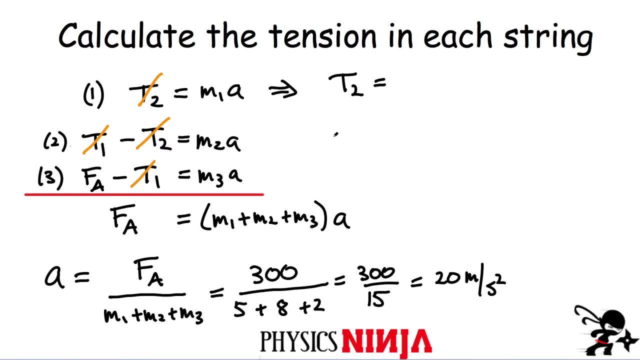 that the tension T2 is equal to the mass M1 multiplied by the acceleration. Well, we just solved for the acceleration. I showed you the quickest way to get to the acceleration. So all you do now is just substitute that value up here. So we have five for the mass and we have our 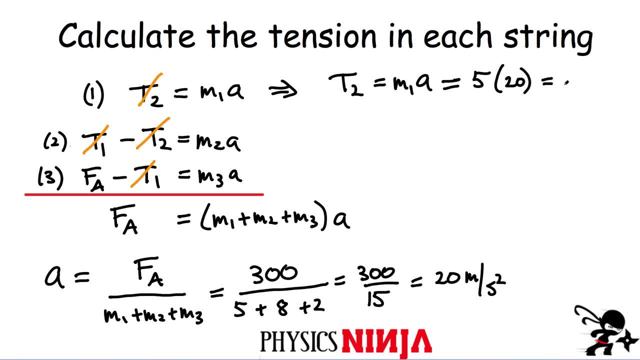 acceleration, which is 20.. Therefore, the tension T2 is simply going to be 100 newtons. So that's the tension between the five and the eight. How do we find the tension T1?? Well, now you can use either equation two or equation three, and you're going to get the same number.